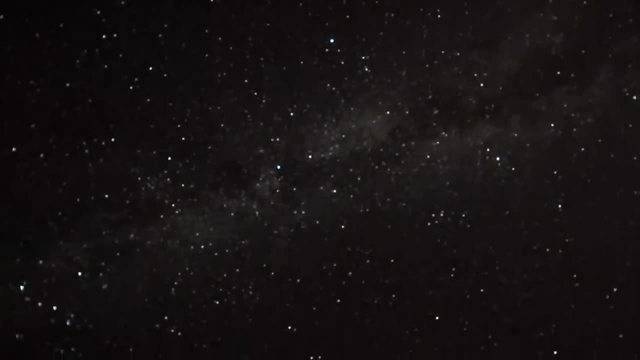 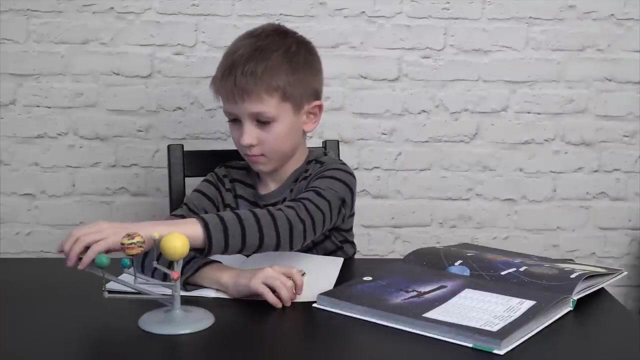 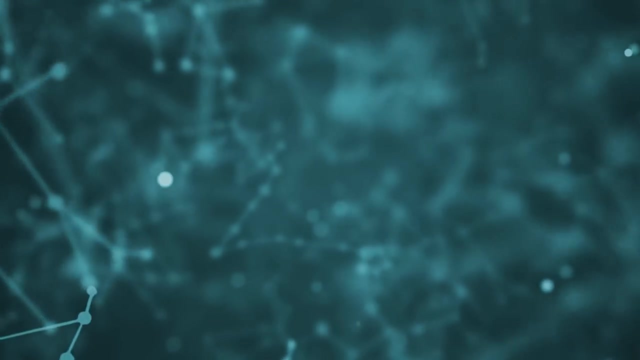 reaches us a star might have been dead for thousands of years already. There are people who study space, stars and the universe for their job. These people are called astronomers. The earliest astronomers noticed that many of the brightest stars in our galaxy formed pictures in the sky. They call these pictures the stars. They call these pictures the stars. 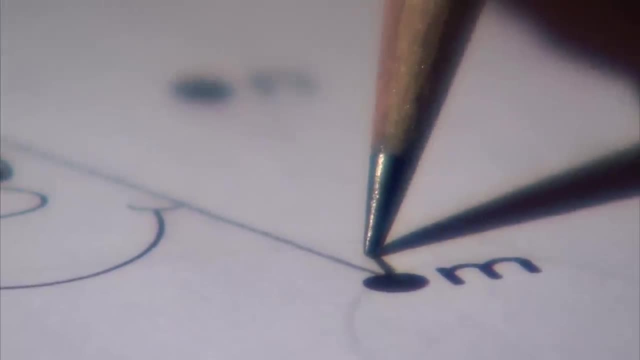 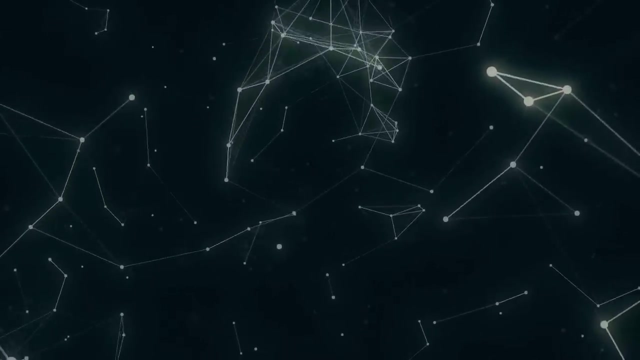 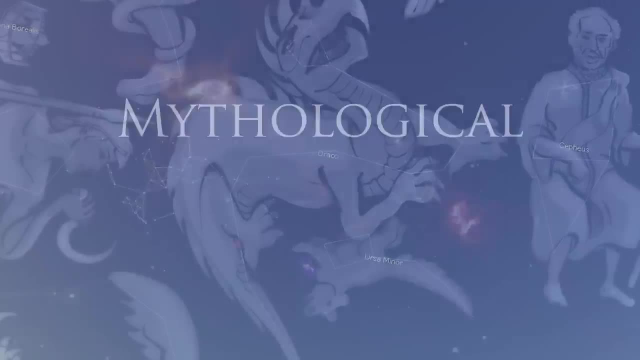 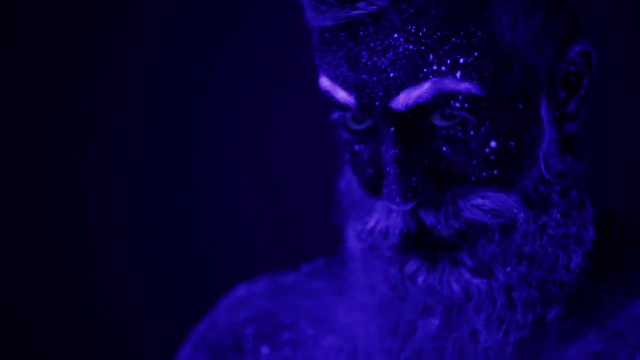 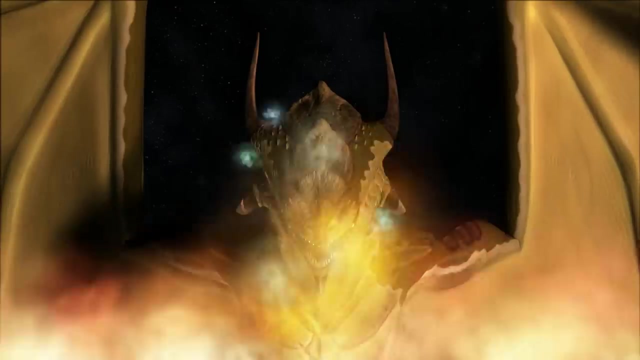 animals and mythological beings. The word mythological comes from the word myth. A myth is a made-up story. The Greeks and Romans made up stories about gods, heroes and creatures such as serpents, dragons or flying horses. They then named various constellations after them. 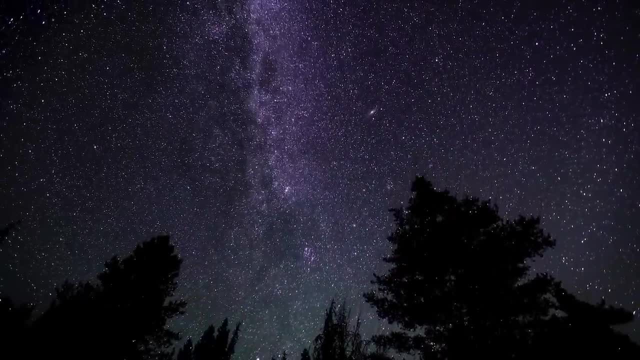 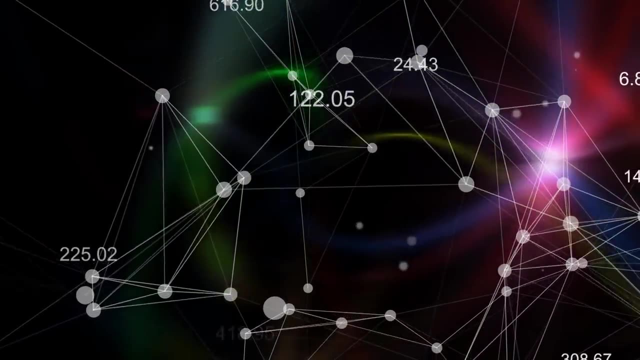 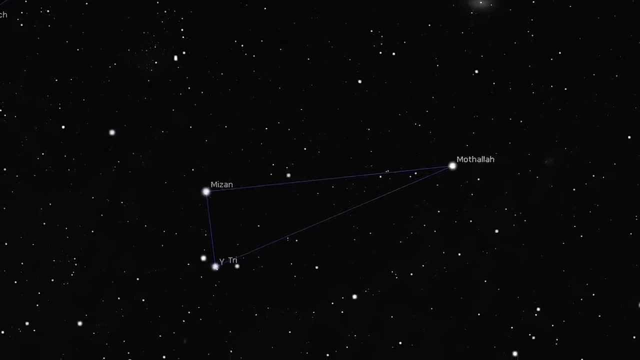 Let's take a closer look at a few constellations that might be familiar to you. As you look at these constellations, you may notice that some of them are easier to see than others. Sometimes the images are just a series of straight lines in a special pattern that may. 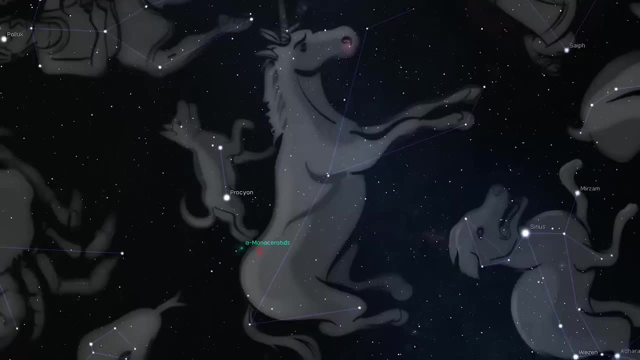 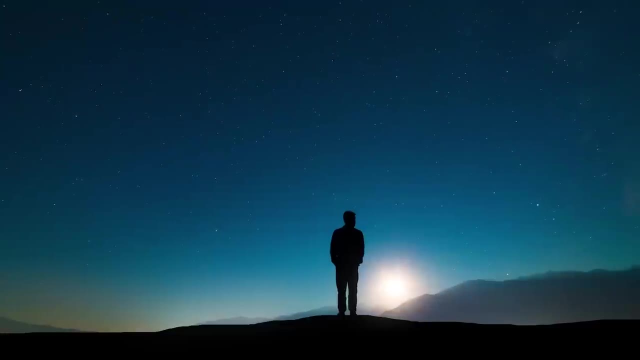 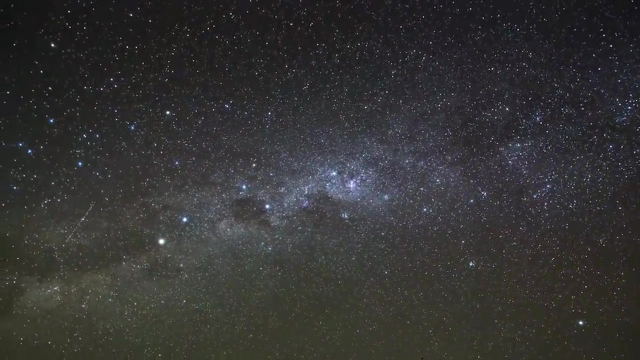 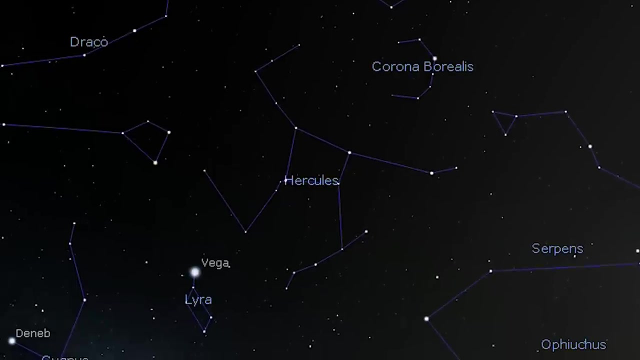 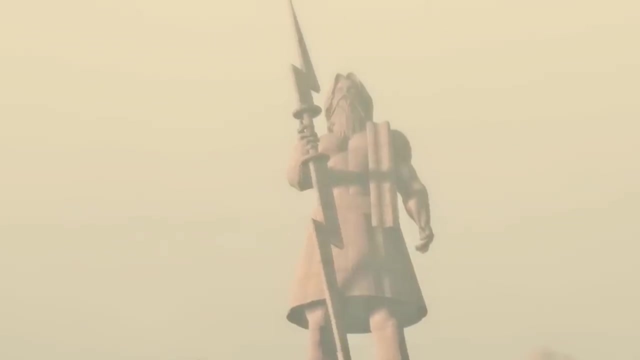 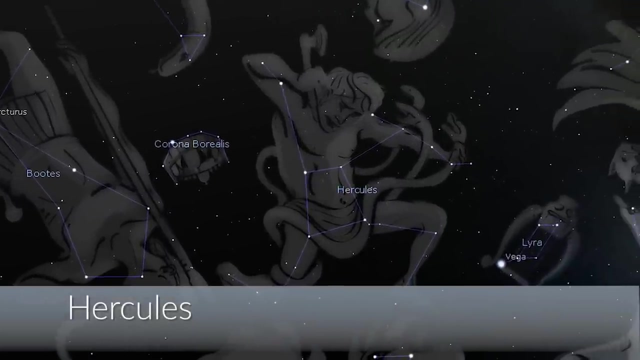 not look exactly like a person, Animal corpse, ensemble, undergroundries and tattooed figures. For instance, those that provide support to women HAVE the right to wear an eye complexion children and was said to be very, very brave. This constellation is an image of Hercules. who became a god after his death. Orion mainly consists of super giant stars, which are the largest and brightest stars. Three of these stars form a line called Orion's Belt. They lead to Sirius, which is the brightest star in the sky. Orion can be seen from both. the southern and the northern hemisphere. From Greek mythology, Orion was a giant and a very good hunter. Zeus placed him among the stars. after Orion's death, Orion looks like he is defending himself from a nearby constellation called Taurus. the Bull Orion is holding a club or weapon in one hand and a lion pelt in the other. 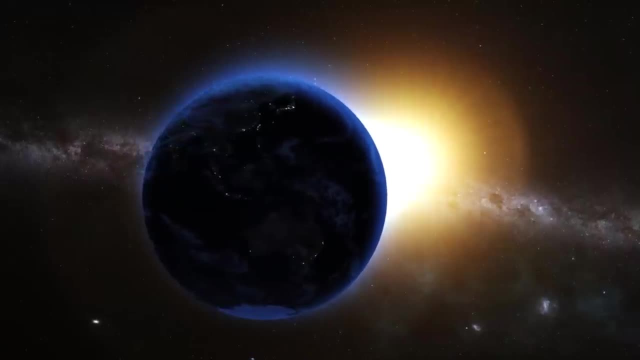 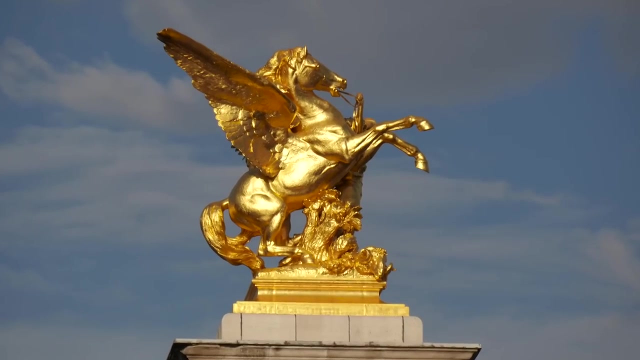 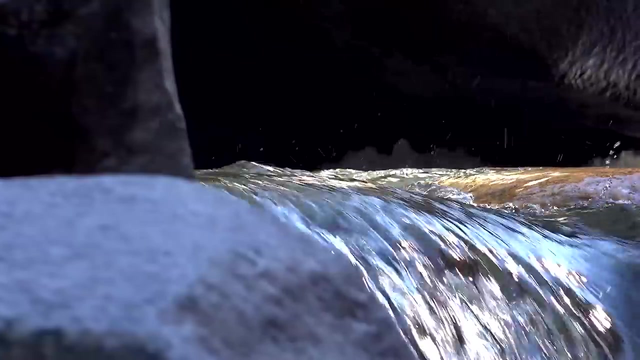 This constellation is visible throughout the world. Pegasus is a constellation in the northern sky. In Greek mythology, Pegasus is a magical horse with wings. One of the stories about Pegasus says that his hooves dug out a spring and anyone who drank the water was given the gift of riding. 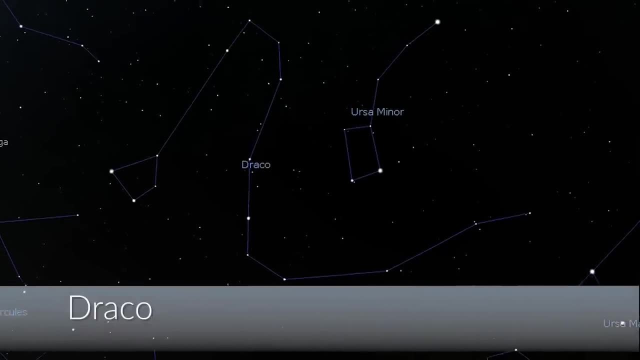 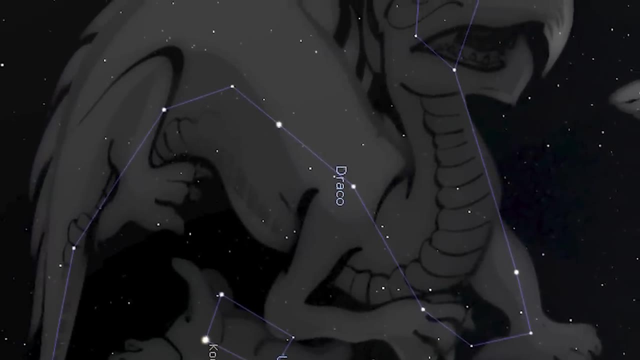 a small walking tree in a spring. The following story is a little more complex than the previous one. This constellation looks like a large snake making its way through the northern sky. It can be seen all year from the northern hemisphere. There are a lot of different myths about Draco. One common myth: 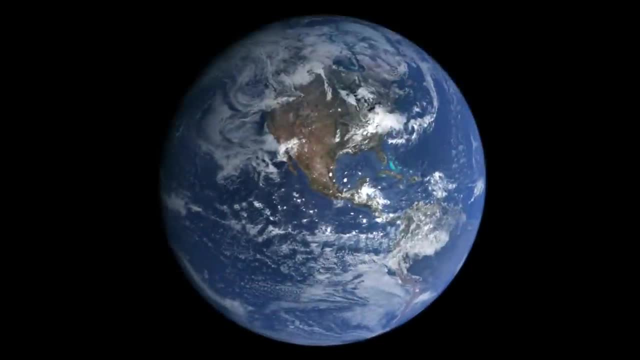 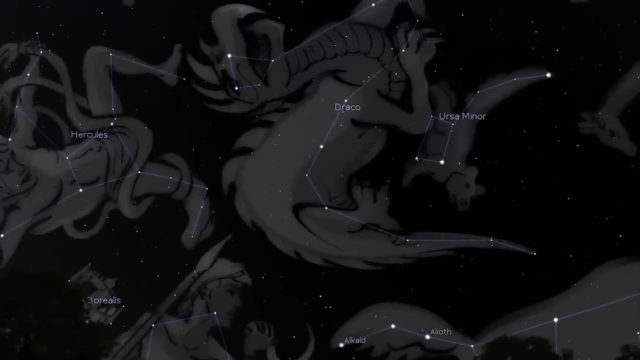 is that Draco was given the job of guarding some golden apples for Hera. The one that Draco was given the job of guarding the golden apple, was given the job of guarding her golden apple. Draco's golden apple is a skull. This is one of the myths that Draco was given for Hera's call to be the guessing. 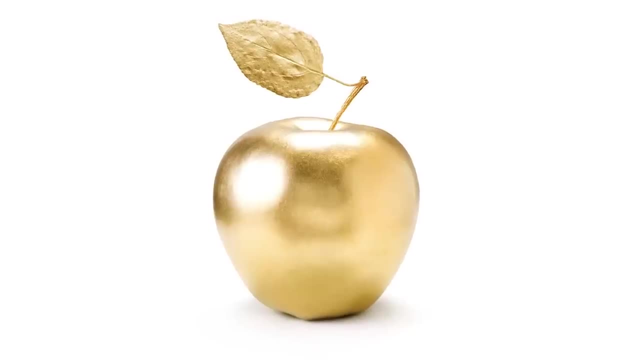 for the golden apples. Draco's skull was the head of the planet. Draco's skull is the voluntary to protect the earth from the 같아서 of Cancer. Draco is the head of the planet. Draco's skull is the. Draco was given the job of guarding some golden apples for Hera, the wife of Zeus. 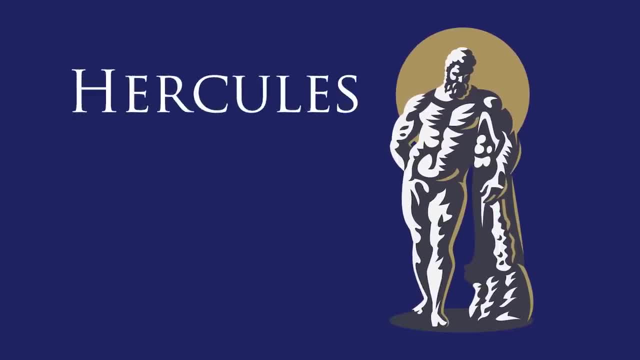 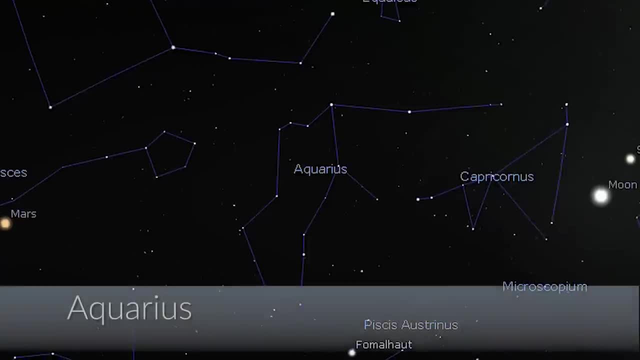 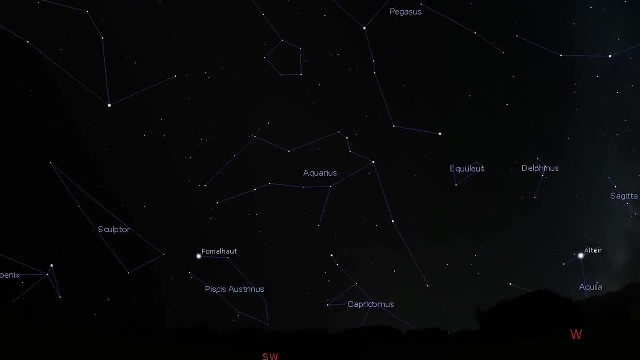 But Hercules slayed Draco to get the apples. Hera was so sad when Draco was killed she placed him in the sky. Aquarius is another large constellation with stars that aren't very bright During different months of the year. it is visible from either the southern or northern. 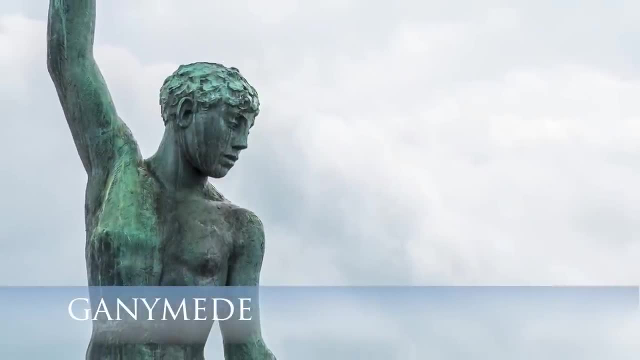 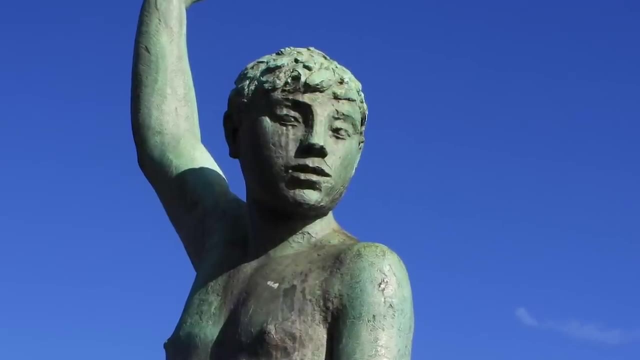 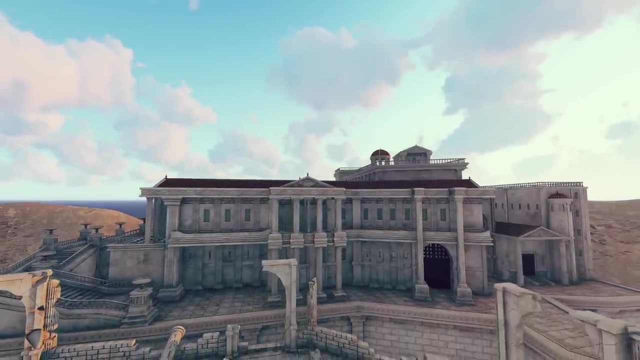 hemispheres. The myth related to the constellation Aquarius is about a man named Ganymede who lived on Earth. Ganymede was very handsome and the king of the gods, Zeus, noticed him. Zeus sent his messenger down to Earth to tell Ganymede to come to Mount Olympus, where the 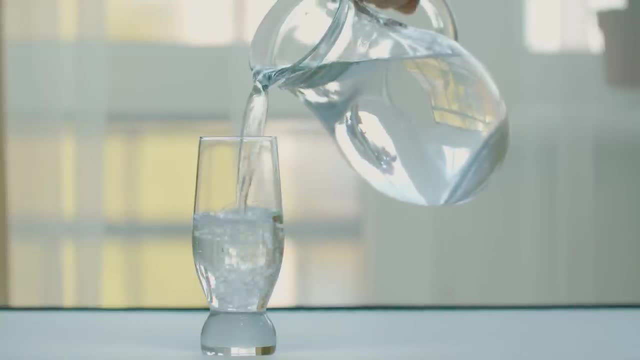 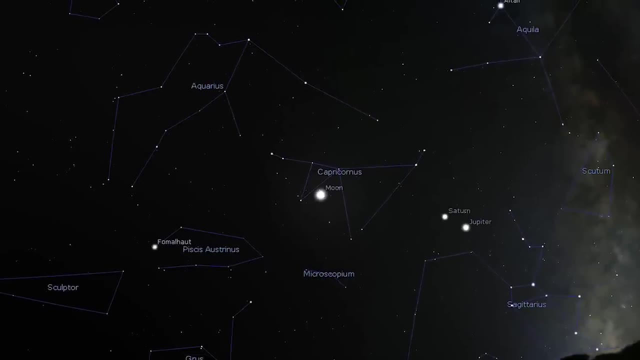 gods lived and serve the gods by bringing them water. Ganymede obeyed. Zeus thanked Ganymede for his service by putting a constellation on Earth. The gods were so proud of him that Ganymede was put to rest in the sky. 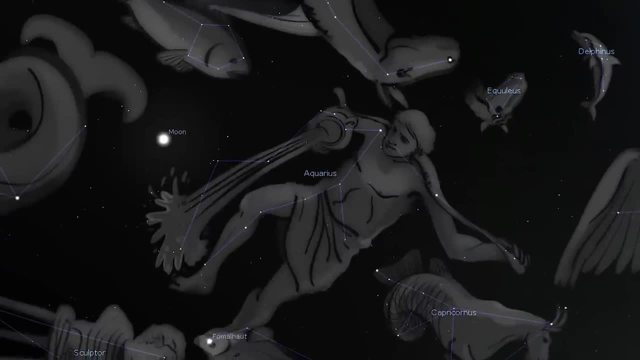 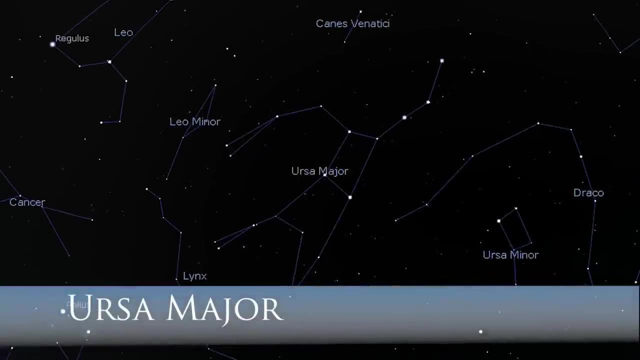 The third constellation is Aquarius. This constellation shows Ganymede kneeling in the sky, pouring water out of a pitcher. The constellation is called the Big Dipper. The Big Dipper is a group of stars inside Ursa Major. Ursa Major means great bear. 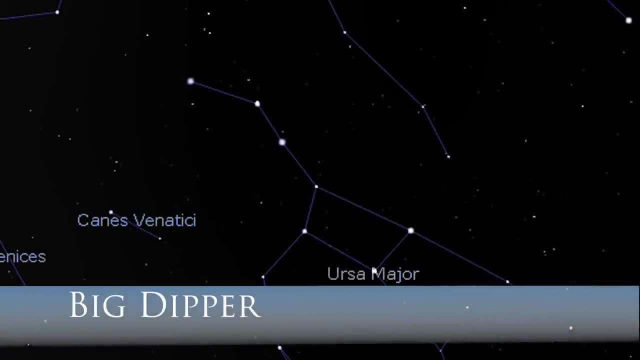 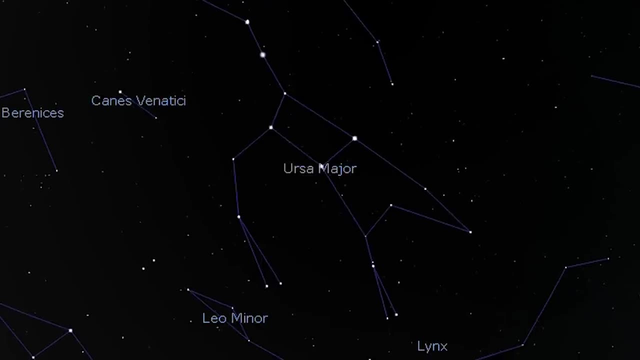 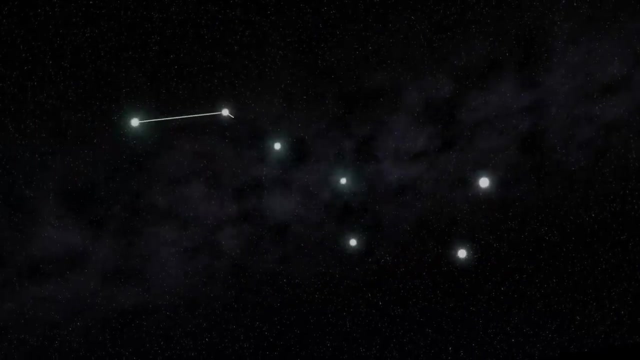 You have probably heard of a smaller section of it called the Big Dipper. The Big Dipper is a group of stars inside Ursa Major. It makes up part of the back half of the bear, the bear as well as its tail. The Big Dipper is not actually a constellation, as some people think. 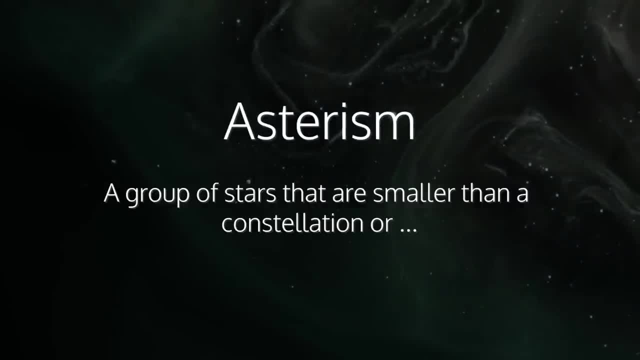 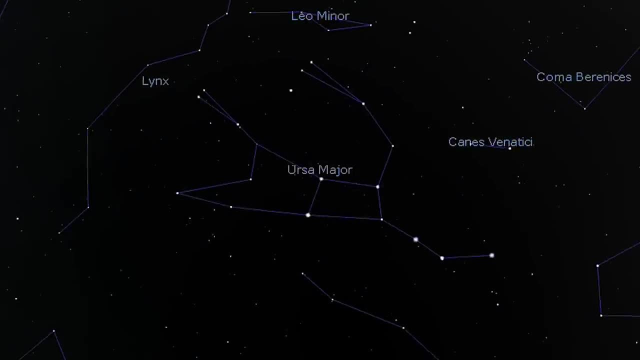 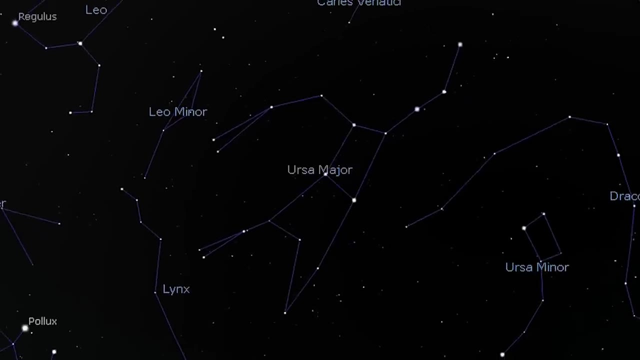 It is called an asterism, which is a group of stars that are smaller than a constellation or are part of a constellation. The story of the great bear is that Zeus turned a beautiful woman named Callisto into a bear to hide her from his wife. Ursa Minor is also known as Little. 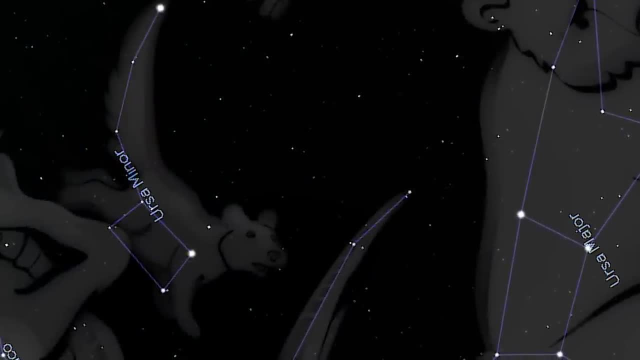 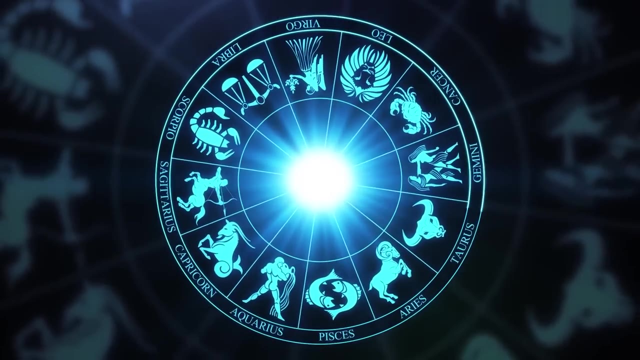 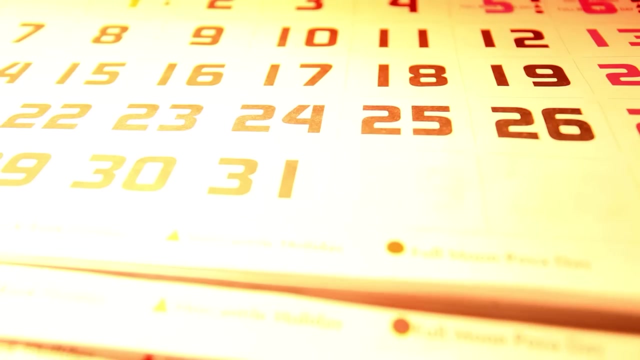 Bear. Little Bear is the child of Great Bear. The Little Dipper makes up part of Ursa Minor. There are 12 other constellations that you also might have heard of called the signs of the zodiac. They represent all the dates in a calendar year. Your birthday determines what your zodiac 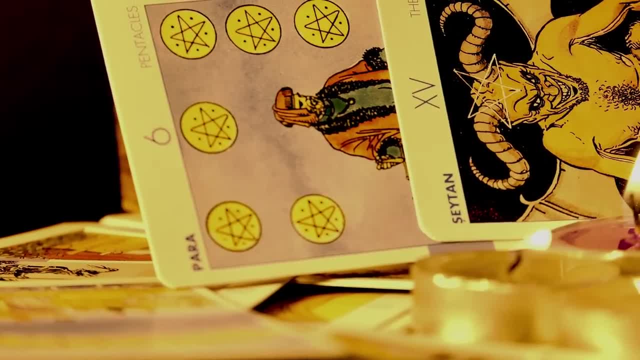 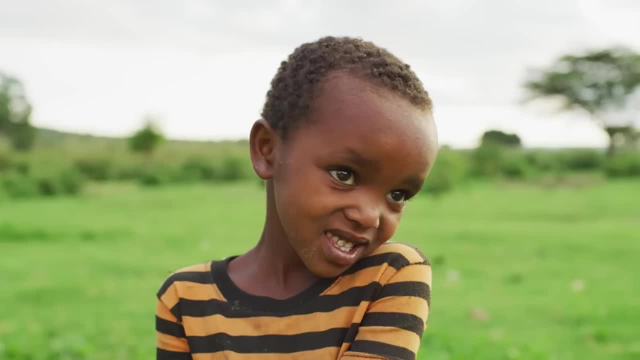 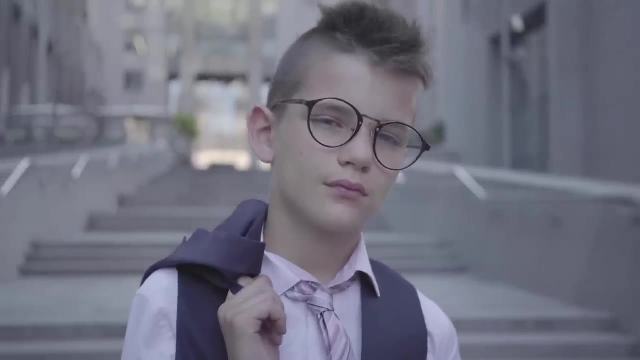 sign is. Some people believe that the different signs of the zodiac will tell you what your time is, Talents are and what your personality is like. The signs might reveal that you are a shy person or outgoing, or that you are laid back or more serious. Some people also believe the signs can 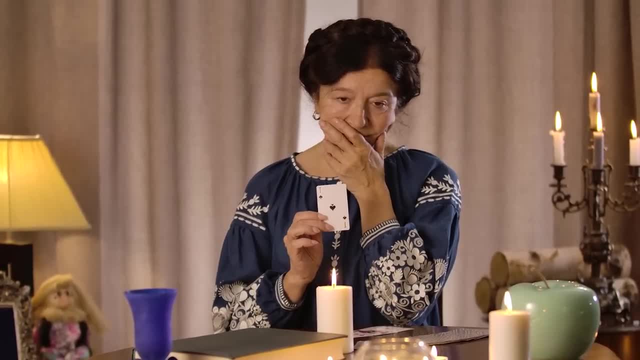 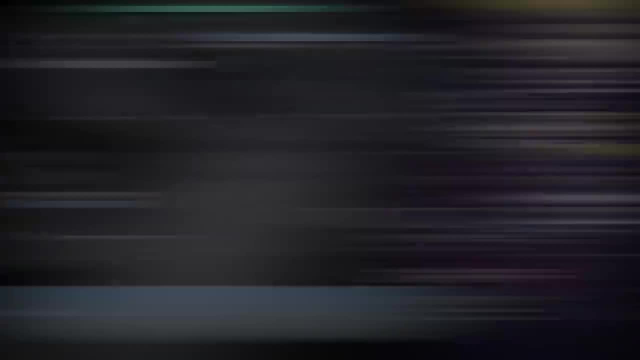 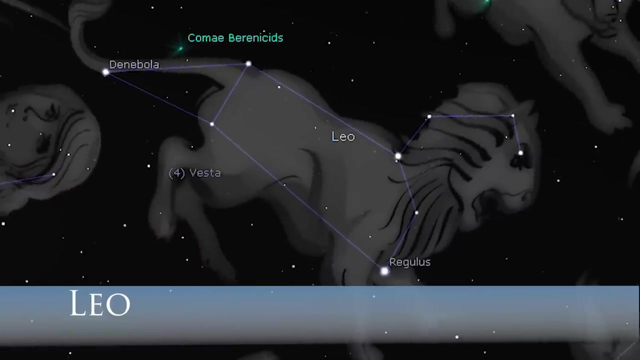 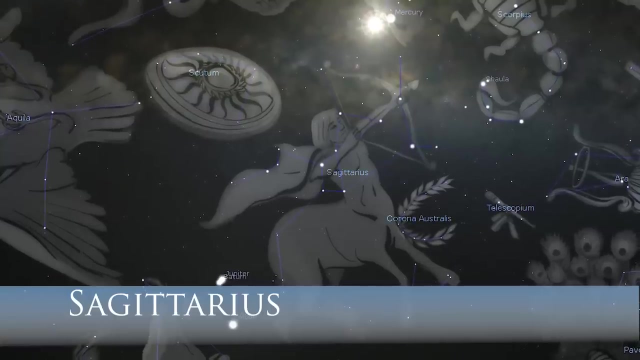 make certain predictions about your life and your future. Here are the locations of the 12 constellations of the zodiac and their names: Aries, Taurus, Gemini, Cancer, Leo, Virgo, Libra, Scorpio, Sagittarius, Capricorn, Aquarius, Pisces. 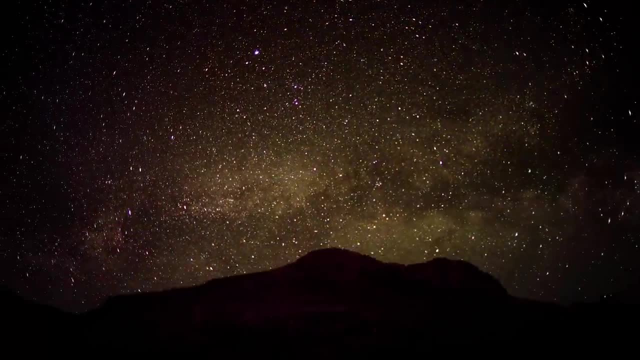 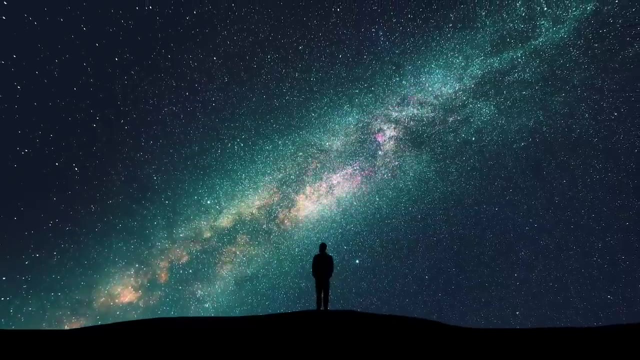 Constellations can be very useful. They have helped ancient farmers know when to plant and harvest crops, and they were used as a type of calendar in the sky. Many travelers relied on different stars and they were used as a type of calendar in the sky Many travelers relied on. different stars and they were used as a type of calendar in the sky. Many travelers relied on different stars like Polaris or the North Star, as well as various constellations, to guide them. other stars like Polaris or the North Star, as well as various constellations, to guide them. 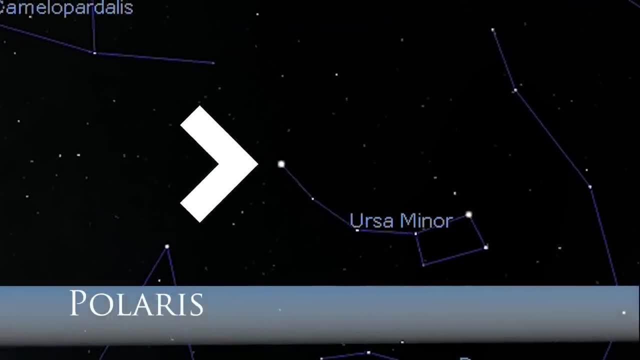 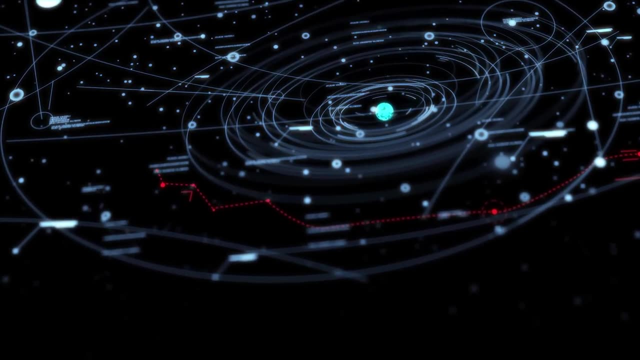 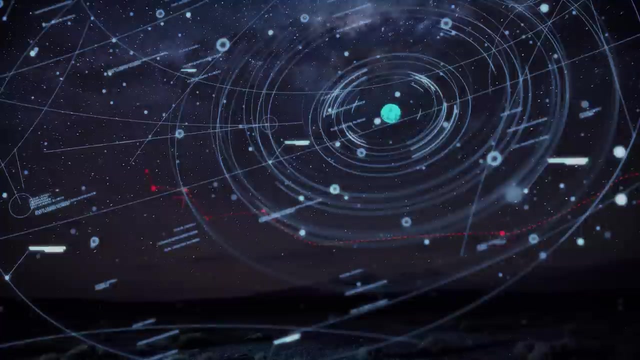 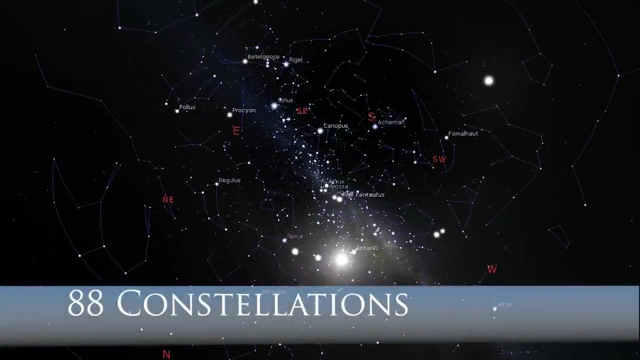 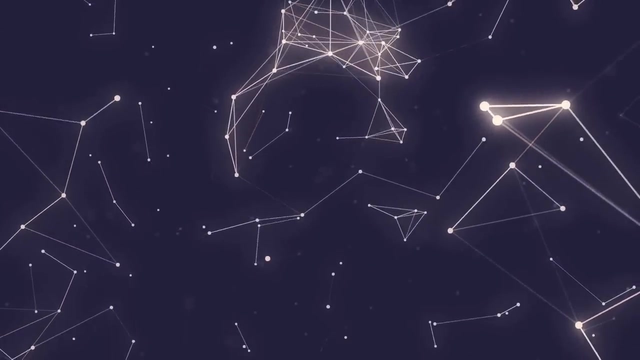 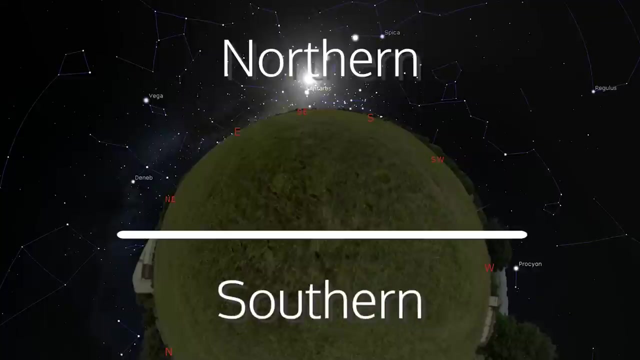 through their journeys. Today, modern astronomers and stargazers use constellations to help keep track of specific Someone. 금 팺 constellations, but not all of them are as well known as others. Many of the constellations may be seen in the northern hemisphere, but may not be. 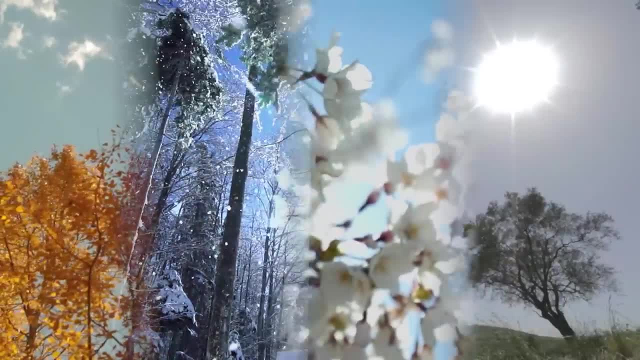 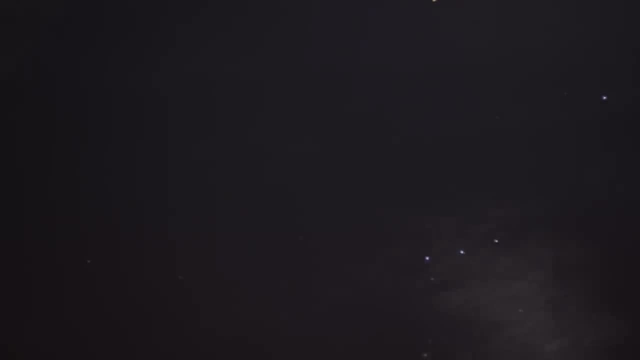 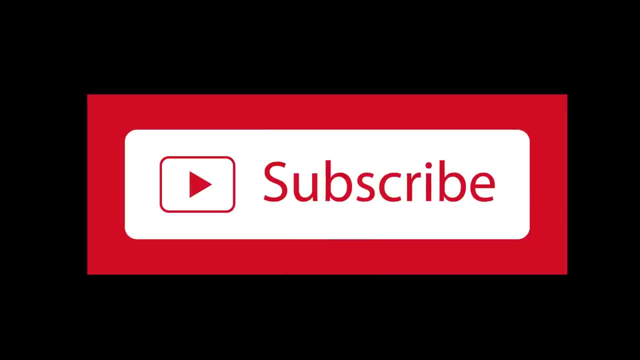 visible in the southern hemisphere, and some may be easier to locate depending on the time of year. The next time you are outside, look up at the stars and see which constellations you can identify. Thanks for following Clarendon Learning. Be sure to subscribe For more free resources. check us out at clarendonlearningorg. 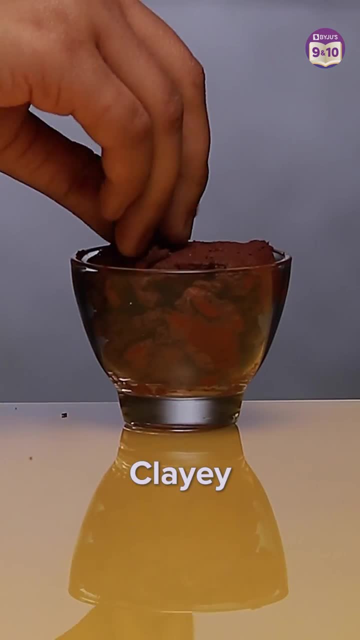 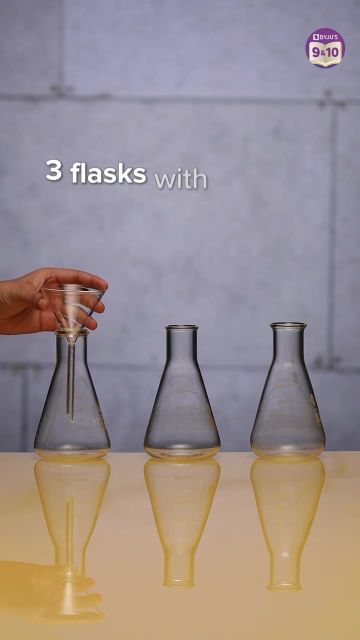 Hey there, Here we have sandy soil, loamy soil and clayey soil with us. Which soil can hold the most amount of water? Let's find out. First take three conical flasks and place funnels in them. Then we plug the funnel with some cotton. 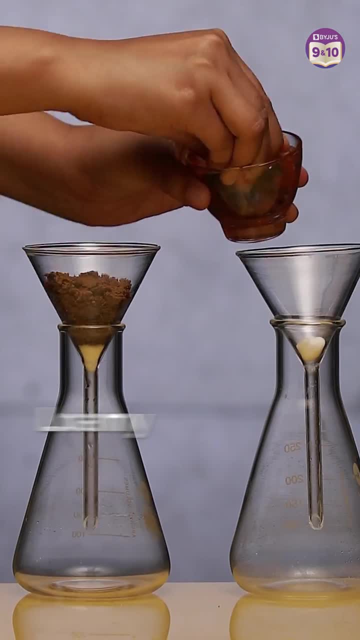 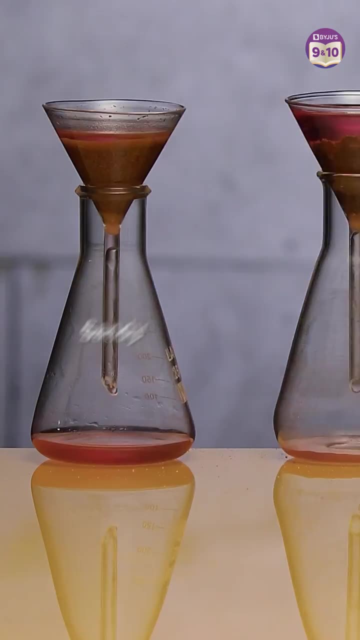 Now fill the funnels with soil and add an equal amount of coloured water to it. Now let's wait for about 20 minutes. Notice the water getting collected at the bottom of each flask. Whoa, There's barely any water in the case of clayey soil. 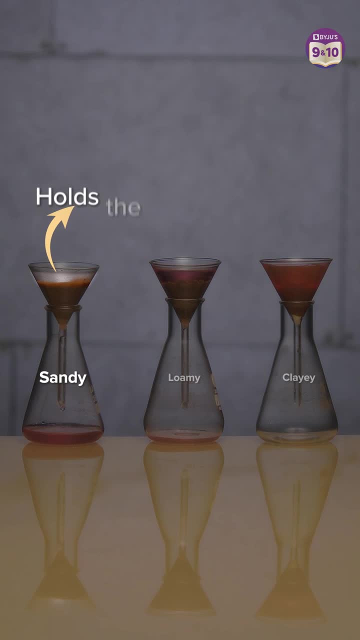 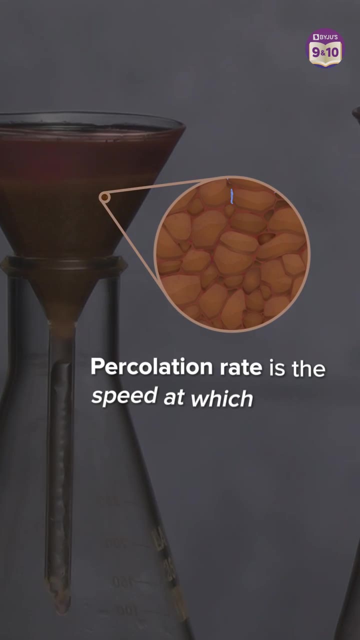 This means that it holds the most amount of water, whereas sandy soil holds the least amount. This happens because of the soils having different percolation rates. Now, percolation rate is the speed at which water moves through the soil. Now, the structure of the soil affects its percolation rate. 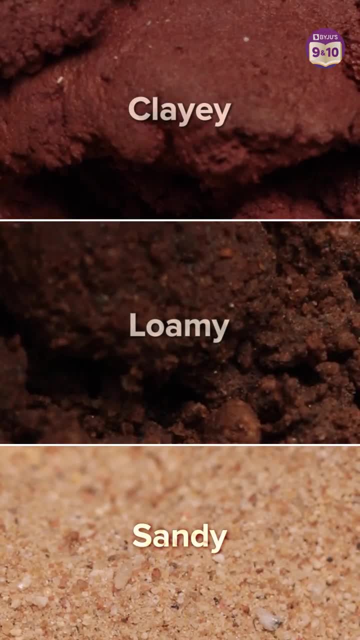 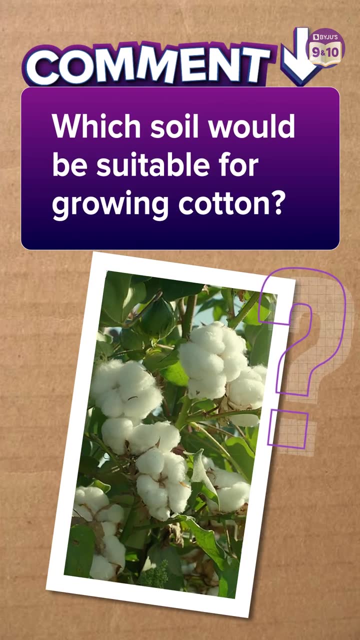 Observe the particle size and structure in these three soils. Because of its tightly packed structure, clayey soil has the lowest percolation rate. Now, which soil can hold the most amount of water? Which soil do you think will be suitable to grow cotton?